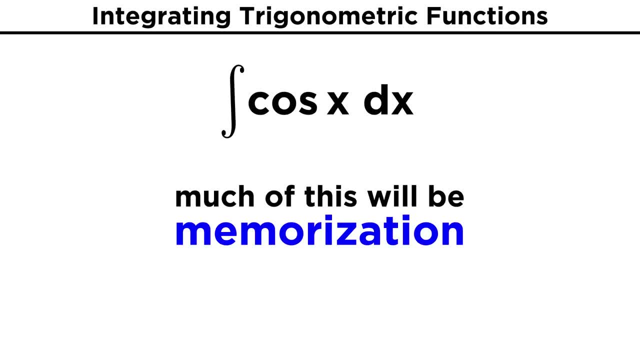 to integrating trig functions, and these will become ingrained over time and with practice. Let's start with cosine x. Earlier, when we discussed differentiation of trig functions, we learned that the derivative of sine is cosine. If this doesn't sound familiar, 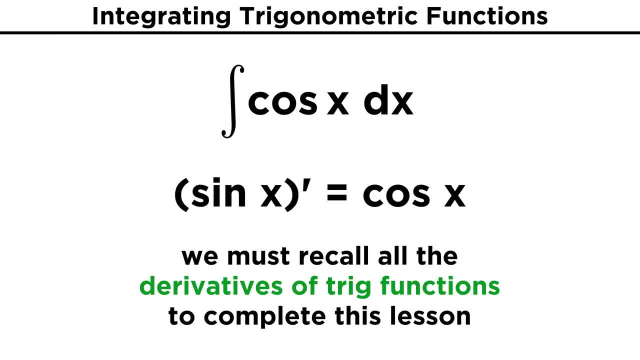 go and check out that tutorial now, because all of the derivatives of trig functions that we learned before will be used here just in reverse. In other words, if the derivative of sine is cosine, then the integral of cosine must be sine. Whatever happens one way, the 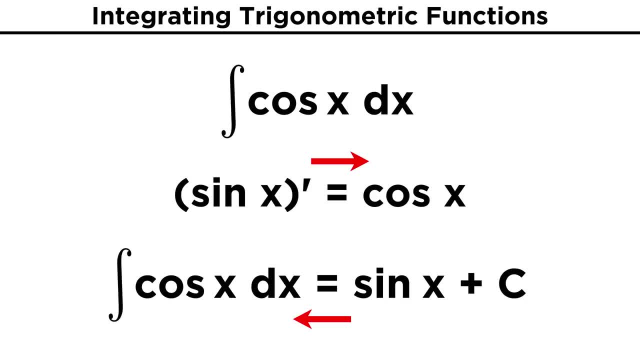 opposite thing happens when we go the other way. And of course, as with any indefinite integral, we must add the constant C. So the integral of cosine x is sine x plus C. We also know that the derivative of cosine is negative sine. so if we need to take the 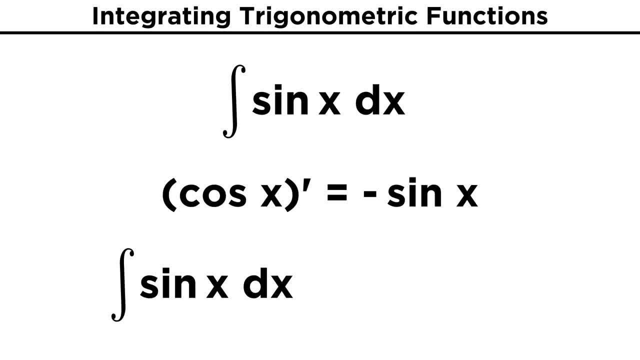 integral of sine x. let's turn it into a form that lists a common derivative simply by writing negative the quantity negative sine x. Then we can pull this first negative outside of the integral, since negative one is a constant, and then integrating negative. 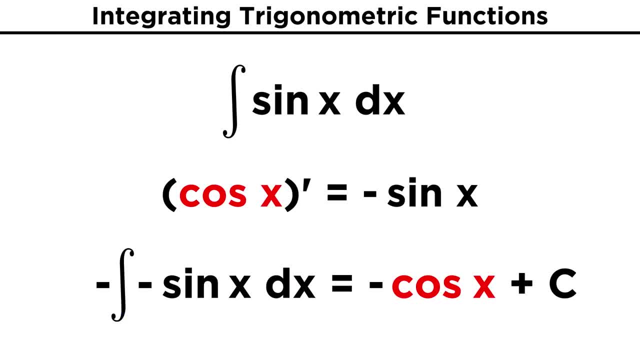 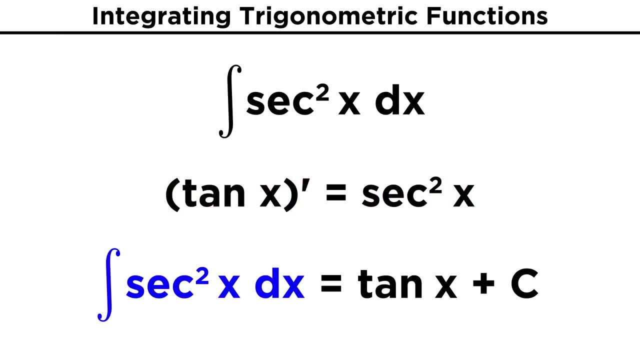 sine gives us cosine. So the integral of sine x is negative cosine x plus C. The derivative of tangent is secant squared. so if we have the integral of secant squared x, that will be tangent x plus C. The derivative of cotangent is negative, cosecant squared. so if we see: 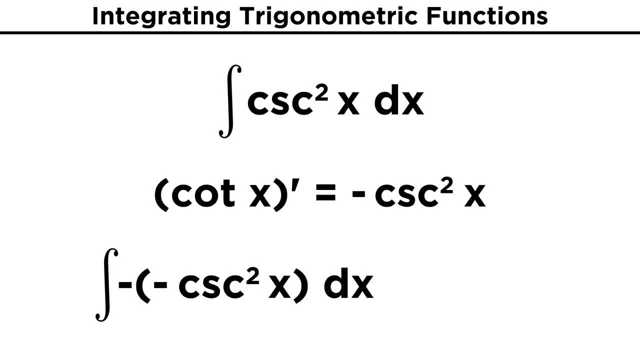 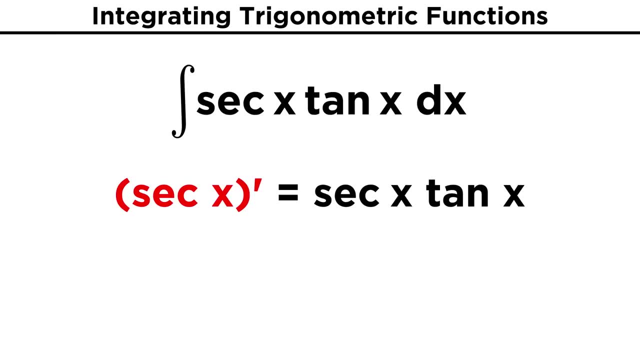 the integral of cosecant squared x plus C. then we have the integral of cosine x plus C. Then we make this the double negative: bring one out of the integral and we end up with negative cotangent x plus C. Then there were the two weirder ones: The derivative. 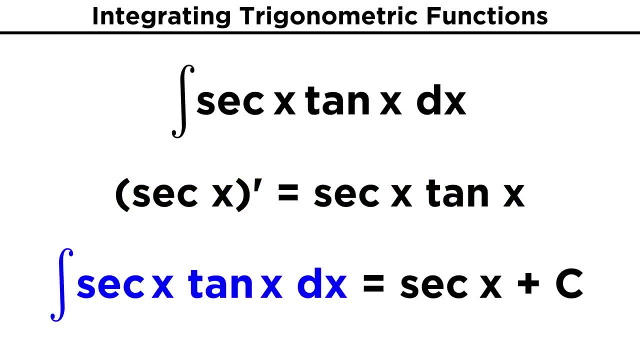 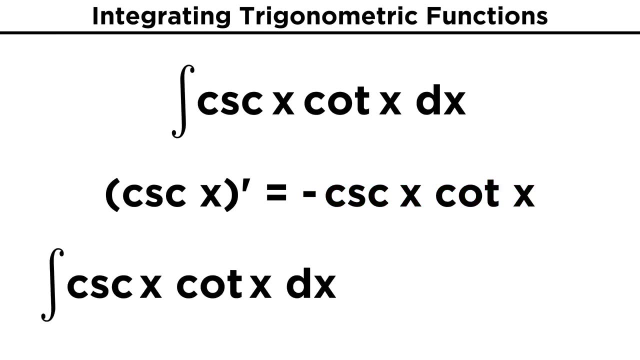 of secant is secant tangent. so the integral of secant x tangent x will be secant x plus C. And then, lastly, the derivative of cosecant is negative, cosecant cotangent. So if we see the integral of cosecant x, cotangent x, we 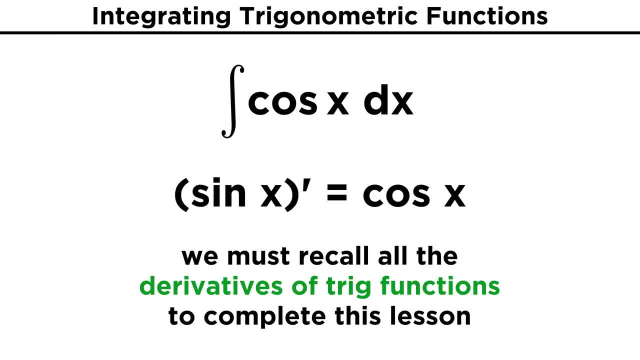 go and check out that tutorial now, because all of the derivatives of trig functions that we learned before will be used here just in reverse. In other words, if the derivative of sine is cosine, then the integral of cosine must be sine. Whatever happens one way, the 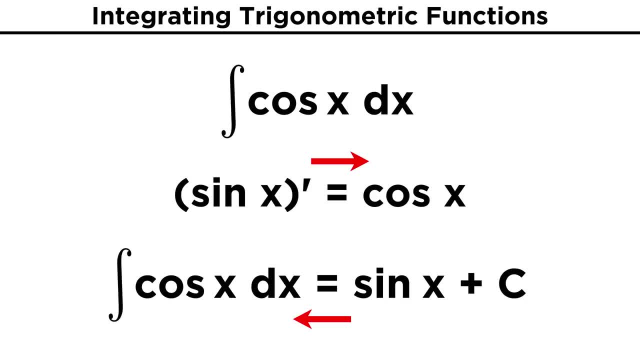 opposite thing happens when we go the other way. And of course, as with any indefinite integral, we must add the constant c. So the integral of cosine x is sine x plus c. We also know that the derivative of cosine is negative sine. so if we need to take the 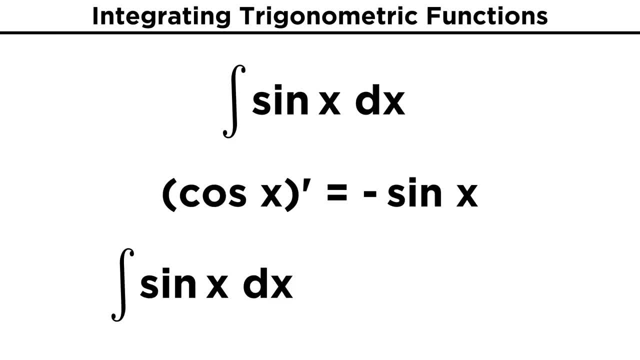 integral of sine x. let's turn it into a form that lists a common derivative simply by writing negative the quantity negative sine x. Then we can pull this first negative outside of the integral, since negative one is a constant, and then integrating negative. 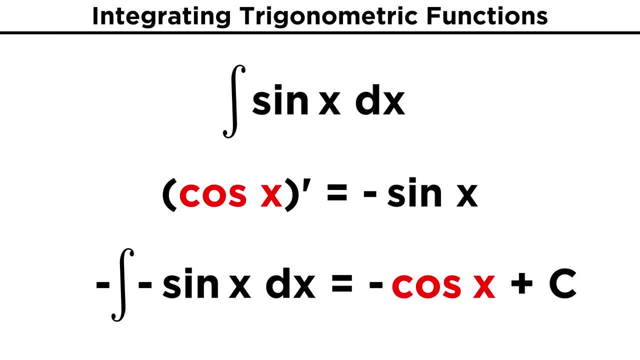 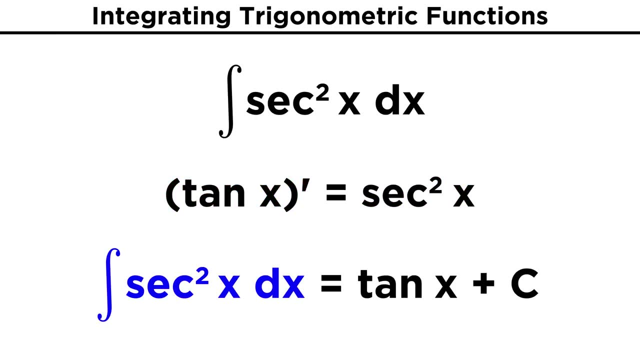 sine gives us cosine. So the integral of sine x is negative cosine x plus c. The derivative of tangent is secant squared. so if we have the integral of secant squared x, that will be tangent x plus c. The derivative of cotangent is negative, cosecant squared. so if we see the integral of cosecant, 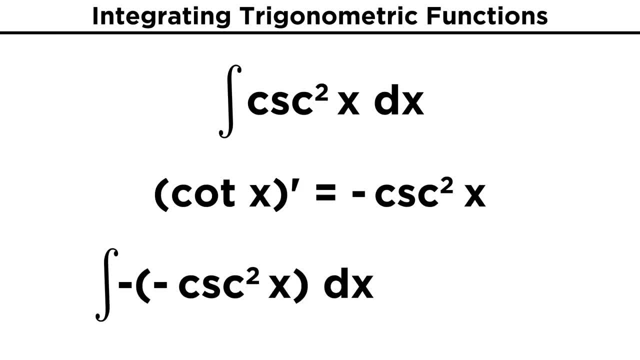 squared x. we'll never know that it's a constant. Thank you for this. questionukearia X. again, we make this the double negative. bring one out of the integral and we end up with negative cotangent X plus C. 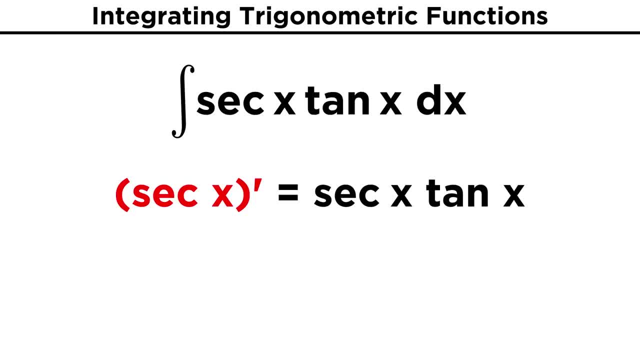 Then there were the two weirder ones. The derivative of secant is secant tangent, so the integral of secant X tangent X will be secant X plus C. And then, lastly, the derivative of cosecant is negative cosecant cotangent. so if we see, 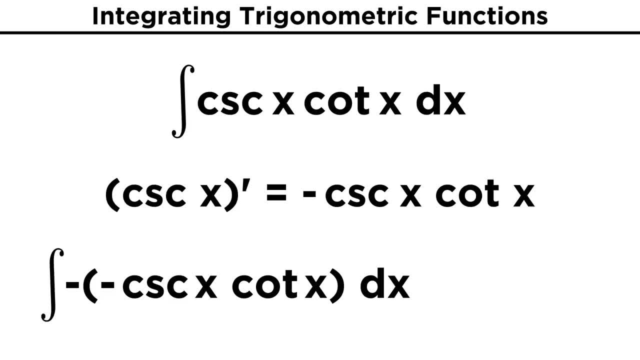 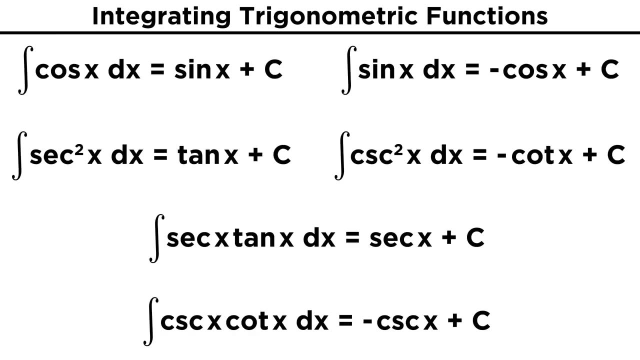 the integral of cosecant X, cotangent X. we do the double negative thing one more time: bring one of them outside and we end up with negative cosecant X plus C. So the good news is that if we have the derivatives of the six trig functions memorized, we don't. 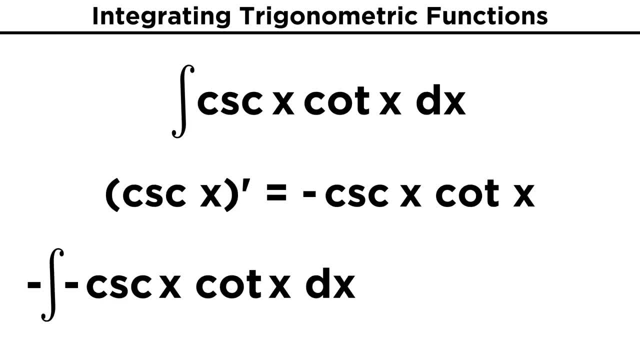 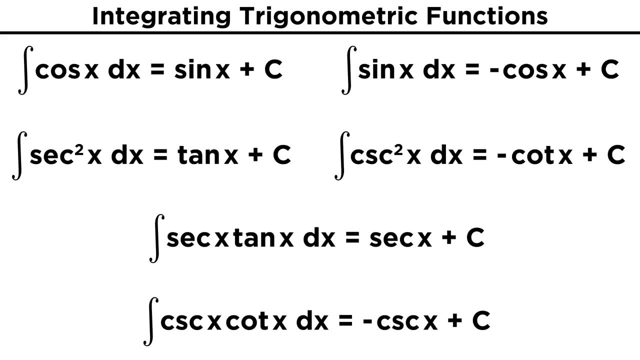 do the double negative thing one more time. bring one of them outside and we end up with negative cosecant x plus C. So the good news is that if we have the derivatives of the six trig functions memorized, we don't really have to learn anything new. We just have to recognize these common derivatives. 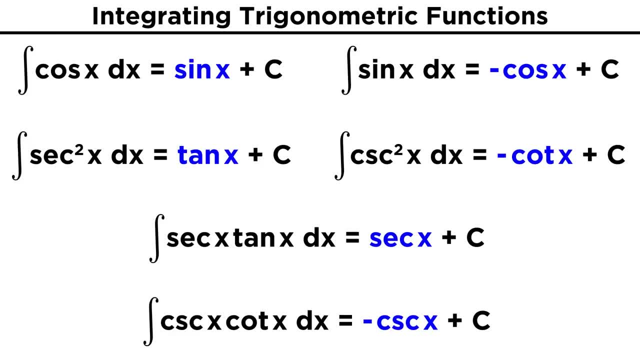 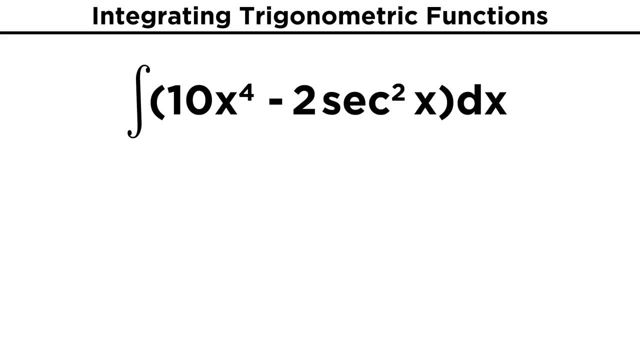 and see them, And then to integrate, we just go backwards to the original function. Let's put this to use. For example: how about the integral of ten x to the fourth minus two secant squared x? Let's make things easy on ourselves and split this difference. 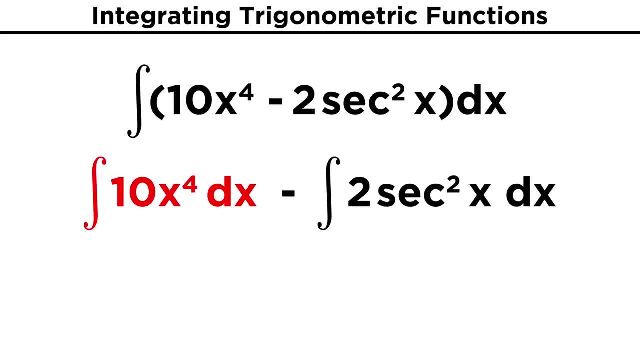 up into separate integrals. The first one is no problem. Ten x to the fourth becomes ten x to the fifth over five or two x to the fifth. Then for the other one we can pull the two out here so that we aren't distracted. 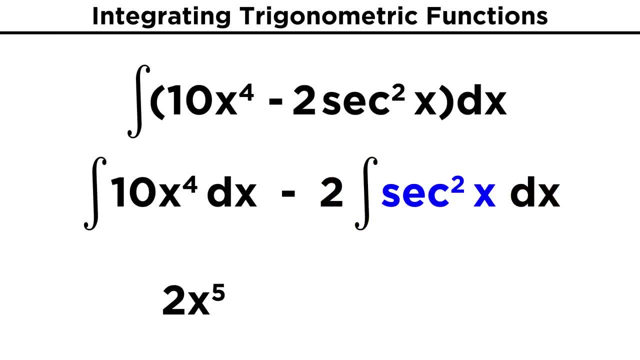 and we can recall that secant squared is the derivative of tangent. so this can become minus two, tangent x, And then finally we finish with plus C. Not too bad, right? Of course, sometimes the common derivative won't just be sitting there for you to spot. You may have to manipulate things. 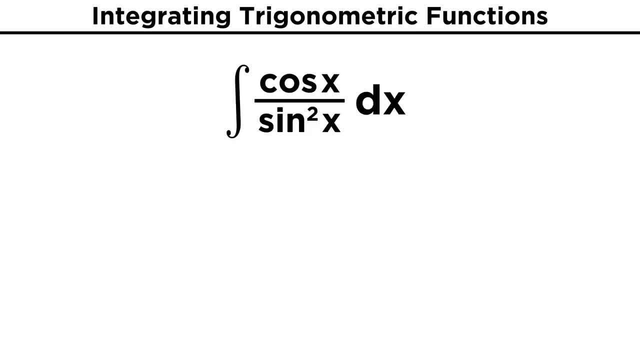 a little bit. How about the integral of cosine x over six? Well, we can do that by multiplying the integral over sine squared x. Again, there is no product rule or quotient rule for integrating, so we can't do anything with this. But when? 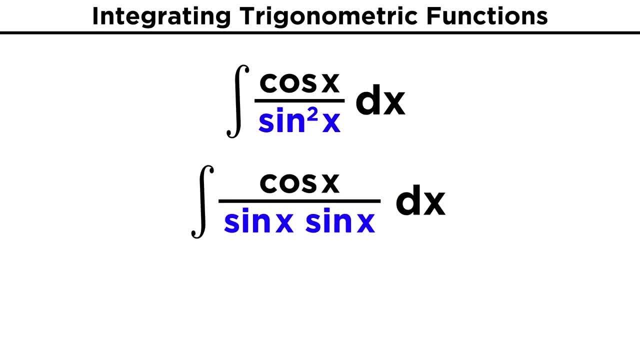 in doubt. just rewrite things in another form and see what happens. What if we write out sine squared as sine times sine? We could then split this into the product of two fractions, one over sine times, cosine over sine. Then we could take: 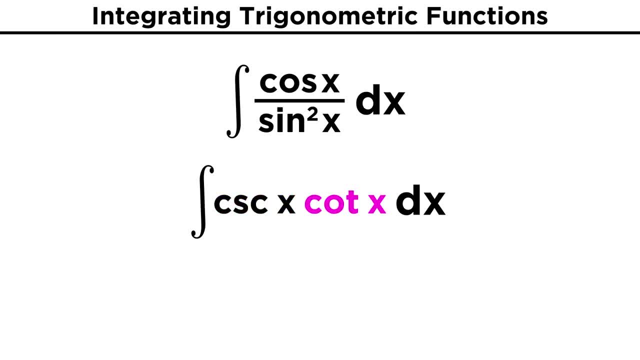 one over sine and turn that into cosecant. and we can also divide that by cosine over sine. also, take cosine over sine and turn that into cotangent. Now we have cosecant x, cotangent x and that is one of the common derivatives we have memorized. 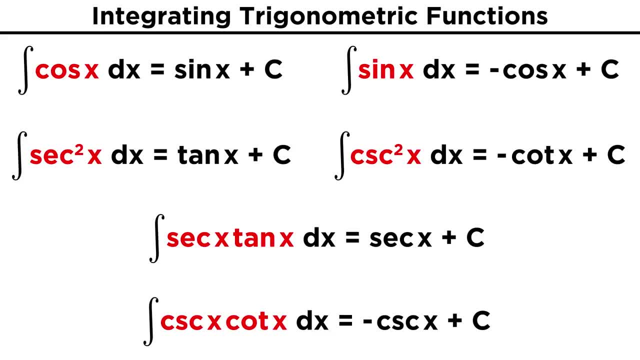 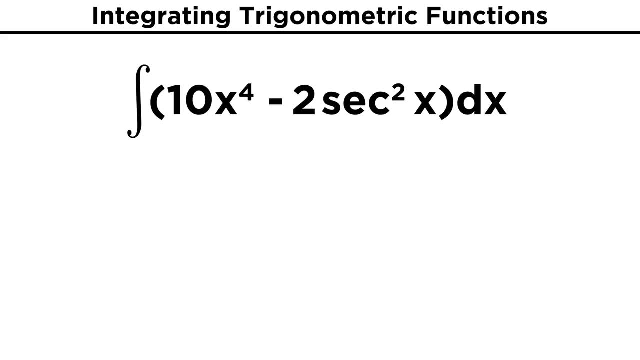 really have to learn anything new. We just have to recognize these common derivatives when we see them, And then to integrate, we just go backwards to the original function. Let's put this to use, For example: how about the integral of ten X to the fourth minus two secant squared X? 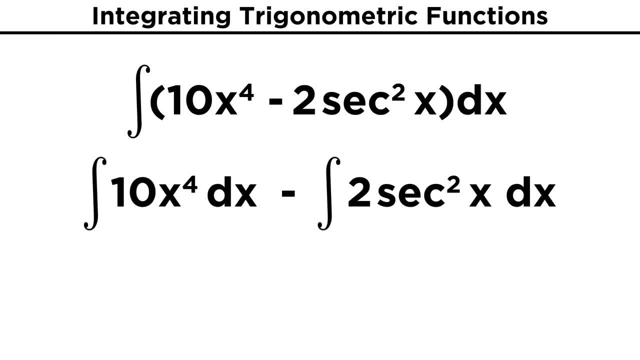 Let's make things easy on ourselves and split this difference up into separate integrals. The first one is no problem. Ten X to the fourth becomes ten X to the fifth over four. So we have the integral of ten X to the fourth minus two secant squared X. 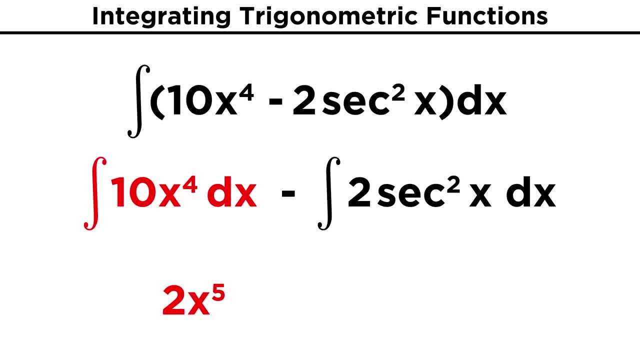 Let's make things easy on ourselves and split this difference up into separate integrals. So we have the integral of ten X to the fifth over four, or two X to the fifth, Then for the other one we can pull the two out here so that we aren't distracted. 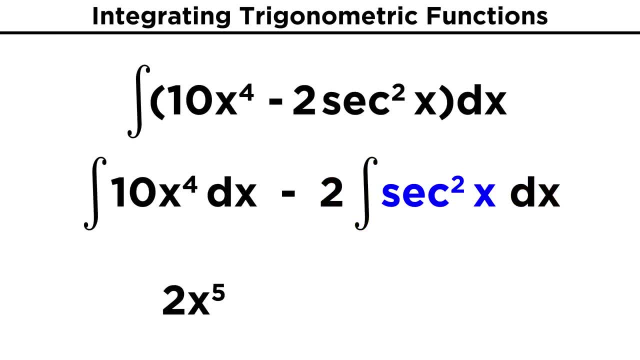 and we can recall that secant squared is the derivative of tangent, so this can become minus two, tangent X, And then finally we finish with plus C. Not too bad right? Of course, sometimes the common derivative won't just be sitting there for you to spot. 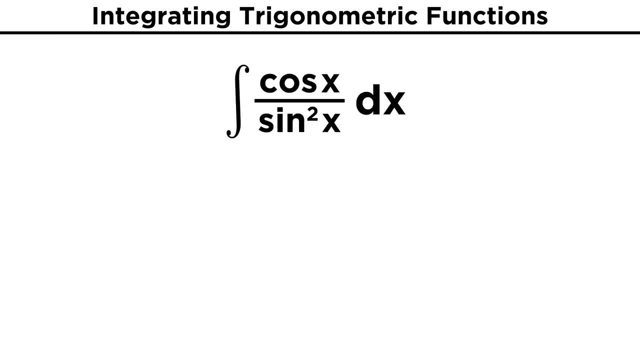 you may have to manipulate things a little bit. How about the integral of cosine x over sine squared x? Again, there is no product rule or quotient rule for integrating, so we can't do anything with this. But when in doubt, just rewrite things in another form and see what happens. 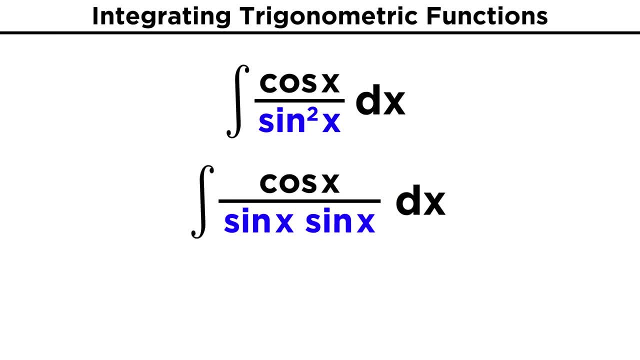 What if we write out sine squared as sine times sine? We could then split this into the product of two fractions: one over sine times, cosine over sine. Then we could take one over sine and turn that into cosecant, and we can also take cosine. 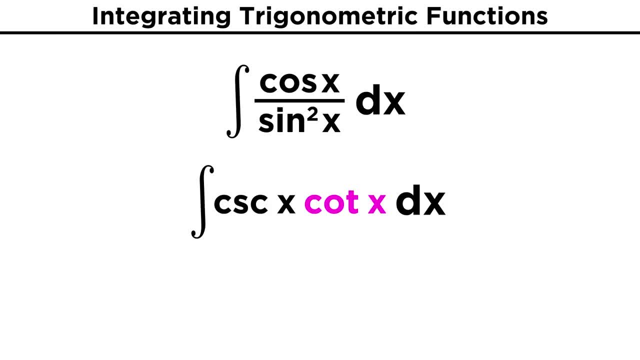 over sine and turn that into cotangent. Now we have cosecant x, cotangent x, and that is one of the common derivatives we have memorized, so this will become negative. cosecant x plus C. Let's do just one more. 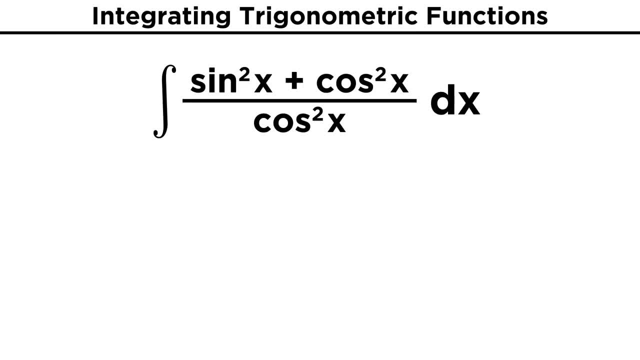 How about sine squared x plus cosine squared x over cosine squared x? Here we are going to have to use one of our trig identities to change things around. Well, we know that sine squared plus cosine squared equals one, so let's make this one over cosine squared, which we know is the same as secant squared.